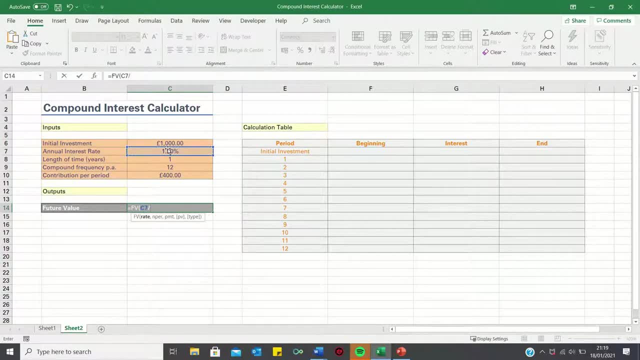 since this is an annual rate, we have to divide it by the compound frequency, which is 12, to give the monthly raise. We then input the number of compounding periods, which is the savings term multiplied by the yearly compounding frequency. We then input the payment. 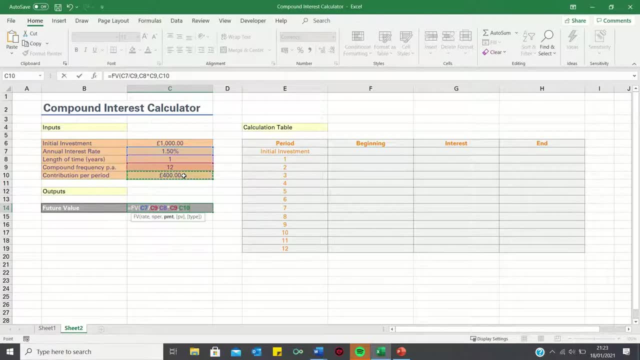 in each compounding period, which is £400,, followed by the initial investment, which is £1000,. and finally, we input 1, because we'll assume that the payment is timed at the beginning of every month. Now, before we click enter, we're going to add: 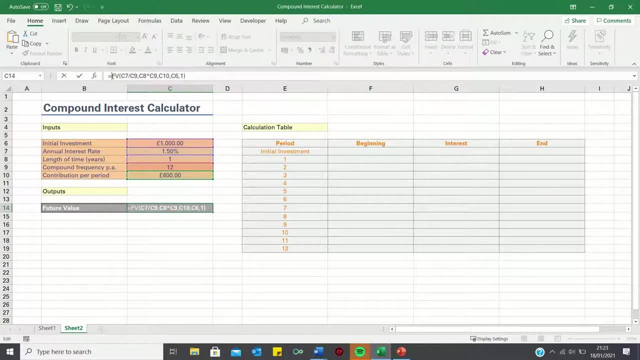 a negative number of compounding periods, which is £1,000, and finally we input 1,, so we can then enter the negative sign in front of the future value formula to ensure that the final value is positive. Therefore, the future value of our savings is £5,854.28.. 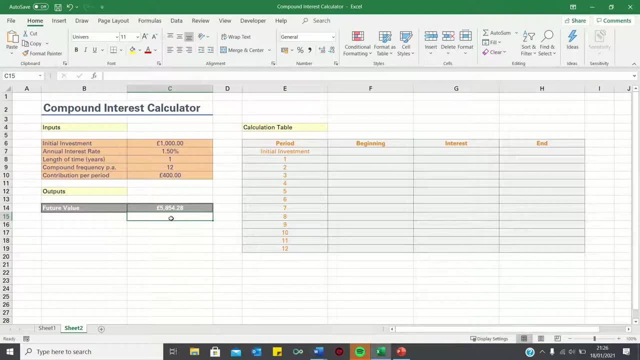 To calculate the interest earned. we can calculate the amount saved without interest, which is £1,000,. so the initial investment plus the monthly standing order multiplied by the number of periods, which is the length of time in years, multiplied by the compound. 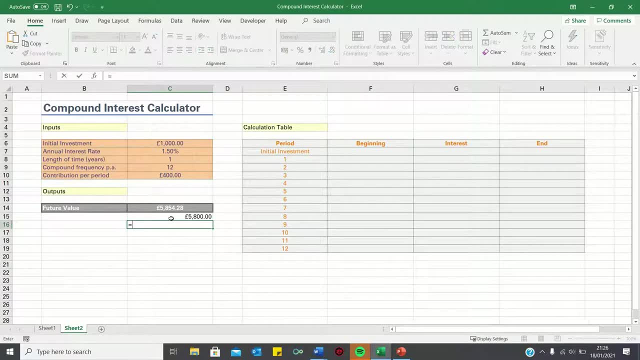 frequency. The interest earned is the future value minus the amount saved. Therefore, this kind of a savings account would earn £54.28 in interest. Now, how do we know that the future value formula calculated the future value correctly? Well, we can build a calculation table to check this. So, for each of the 12 months or savings, 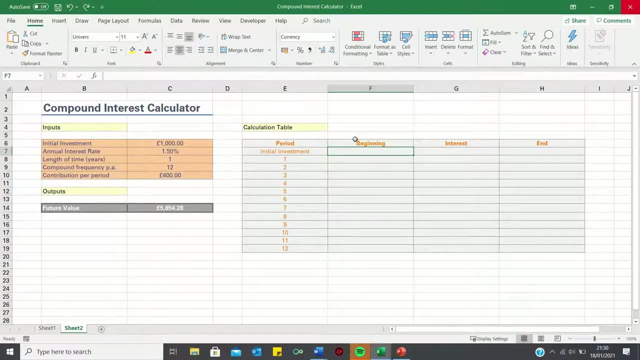 periods. we're going to calculate the amount in the account at the beginning of the month, the interest earned and the amount at the end of the month. Initially, the amount in the account will be £1,000, which is the initial investment, The interest payment at. 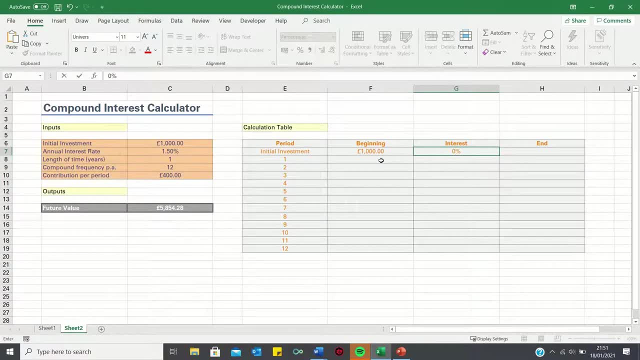 the start will be 0%, as we'll only be earning interest in months 1 to 12.. Our amount at the end is the initial investment multiplied by 1, plus the interest rate, which stays the same. as the interest is 0% In month 1,, we'll have the amount at the end of the previous. 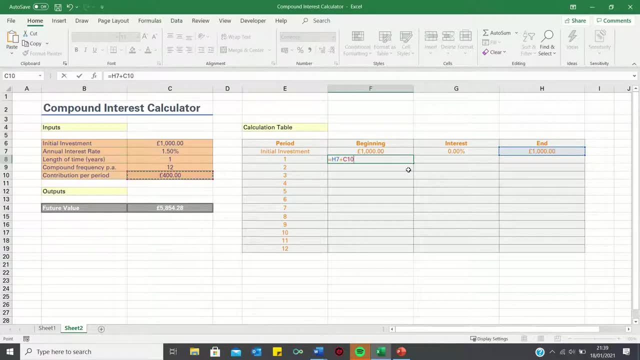 month plus our monthly contribution. Before we click enter, we're going to add absolute references to ensure this value remains static as we bring it down later. The interest earned in months 1 to 12 is the annual interest rate, which is 1.5% divided. 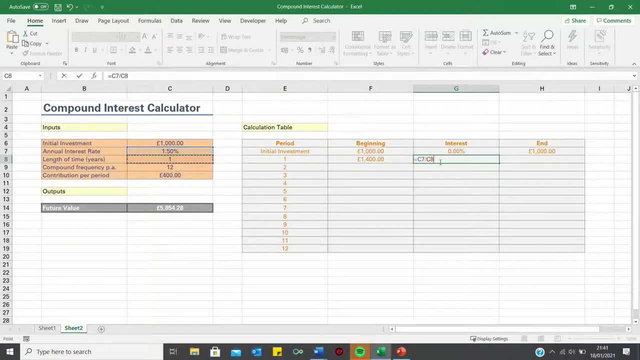 by the number of compounding periods, which is 12, to give the monthly rate. Now, once again, before we click enter, we're going to add absolute references to both of these and ensure they remain static. Our savings amount at the end of the month is the amount at the start of the month multiplied. 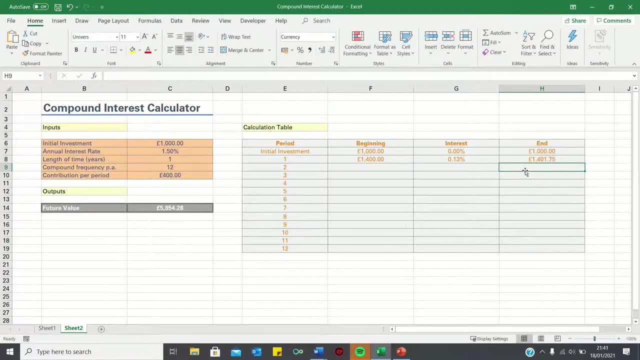 by 1 plus the monthly interest rate. Therefore, at the start of the month, we'll have £1,400 in our accounts and we'll have earned an interest of 0.13%, which will grow our savings by £1.75.. Now to bring these formulae down to the remaining months, we can simply select. 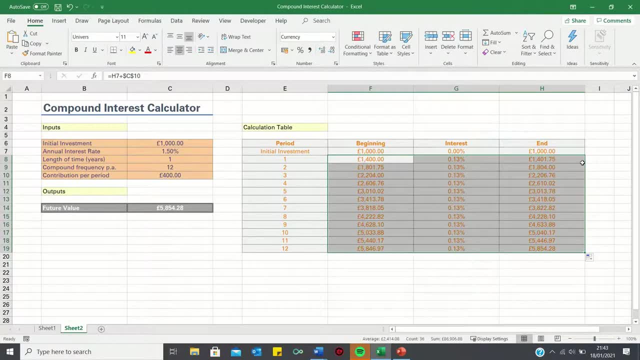 this row and then double-click the bottom right-hand corner. This has calculated the amount at the start and end of all 12 months. As you can see, the amount at the end of month 12 is the same as the future value we calculated earlier. 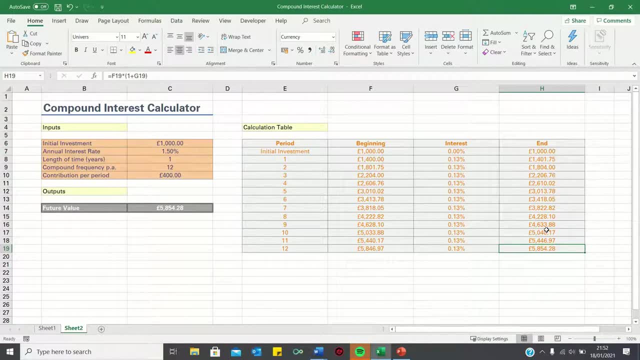 Now we can test whether the values still match when using different figures. So let's change the initial investments, the interest rate and the monthly contribution Once again. both figures match. Now, if we change the term to two years instead of one year, you'll notice that the figures no longer match. This is because our calculation table 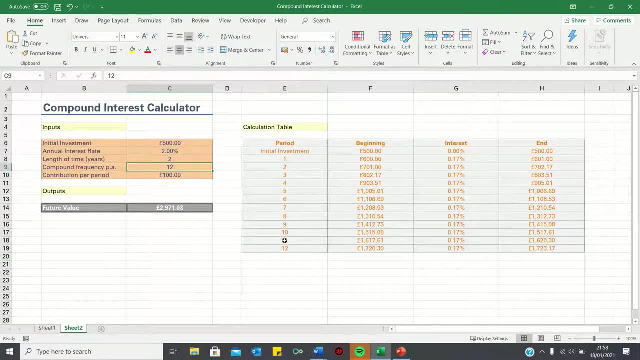 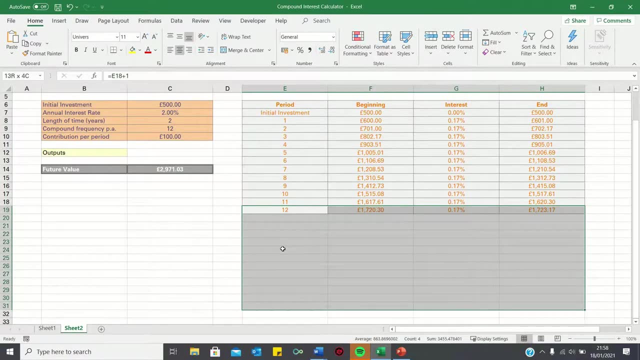 is still only considering 12 months or 1 year. To make the figures match, we'll have to drag the calculation table to calculate 24 months or 2 years. As you can see, now both figures match. So that's how you can create a compact account. 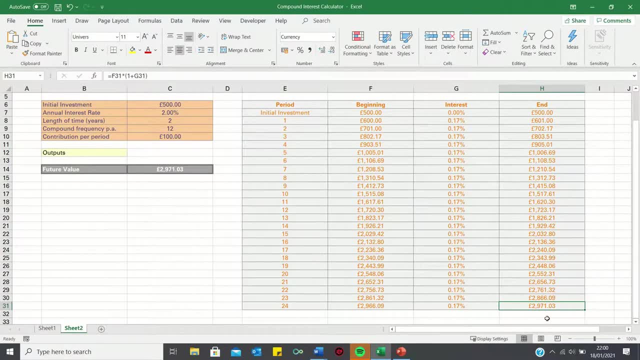 Please comment down below if you have any questions. give this video a thumbs up if you found it useful and subscribe to the Excel Hub for weekly Excel tutorials, techniques and examples.